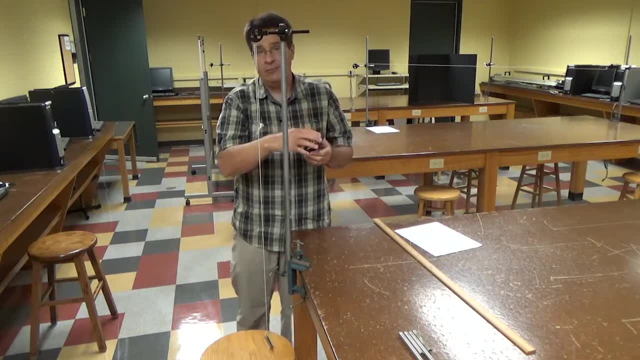 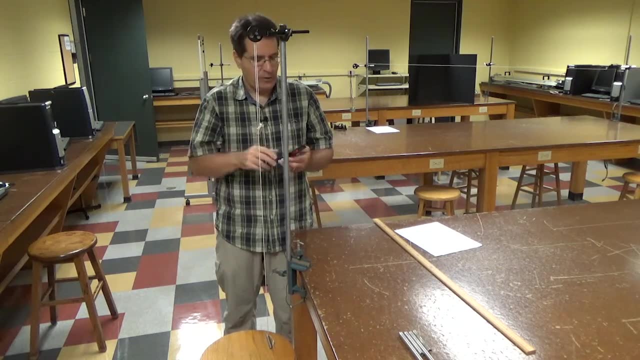 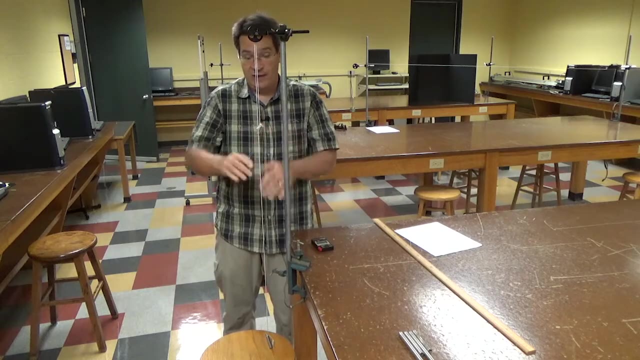 So when you get your raw data you'll have three times, because we would do this three times in lab because of timing error or any other uncertainties. You'll be given three raw times, you'll take an average time and knowing that average time and that height difference, 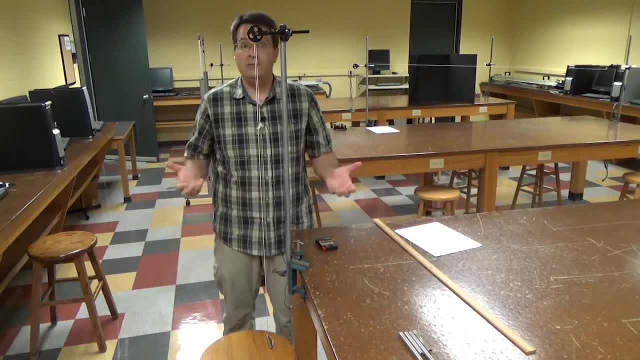 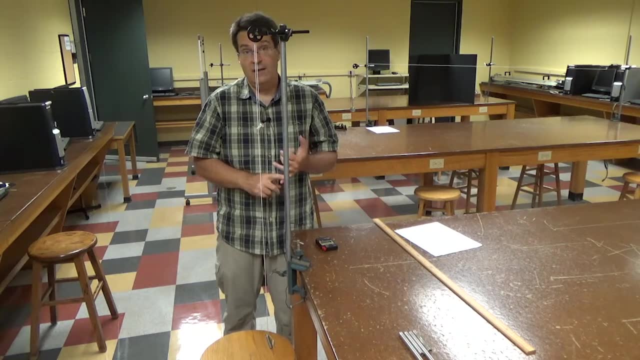 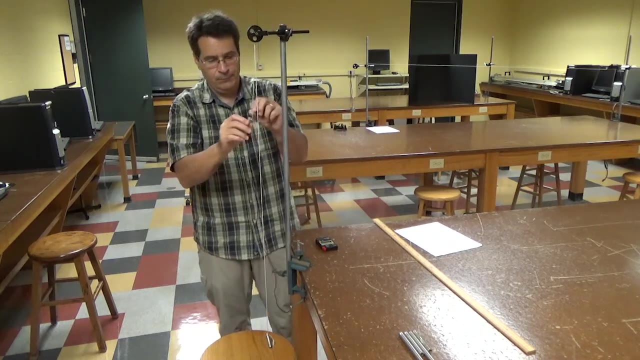 of 100 centimeters which you'll be given. we can then do the analysis, lots of analysis, using both force and acceleration, Newton's second law, but also an energy analysis. Now you'll be given data for the 40 gram, 50 gram machine. 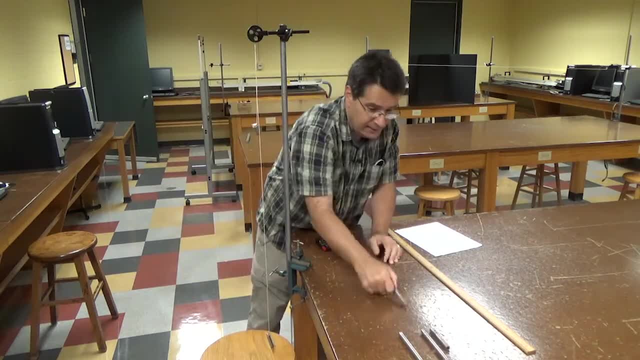 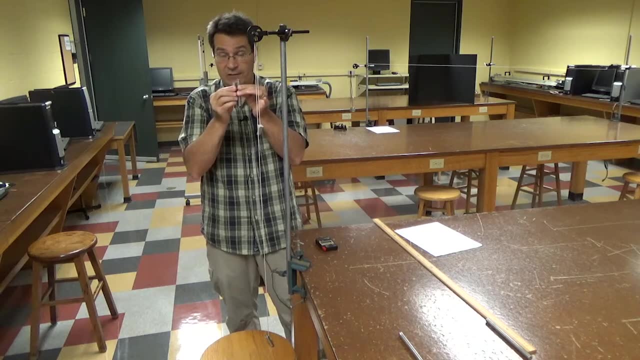 You'll also be given data for a 90, 100 gram machine. Okay, the 90, 100 gram machine. notice, it's still 10 grams of difference, of difference, of difference. Do you see any difference between the two sides? 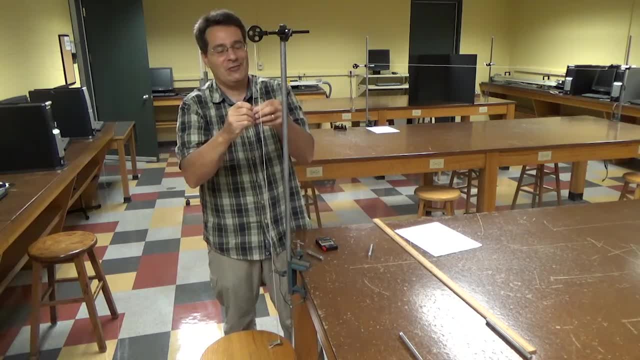 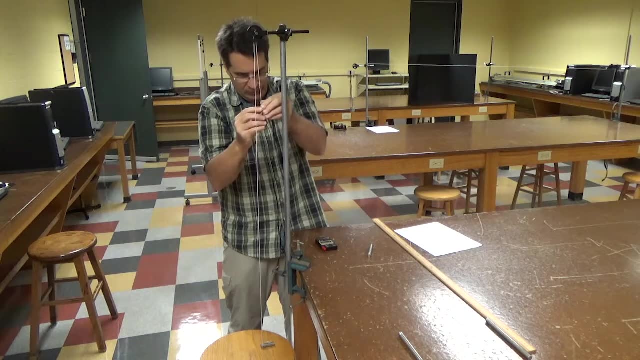 Let me just see if I can get this set up for you. I'm going off script now. Yup, you can see that I'm definitely going off script. Okay, so here's the 90, but I wanna show you something experimentally. you would see if you were doing this lab. 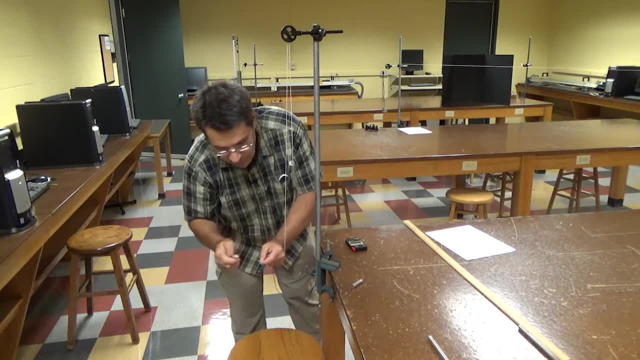 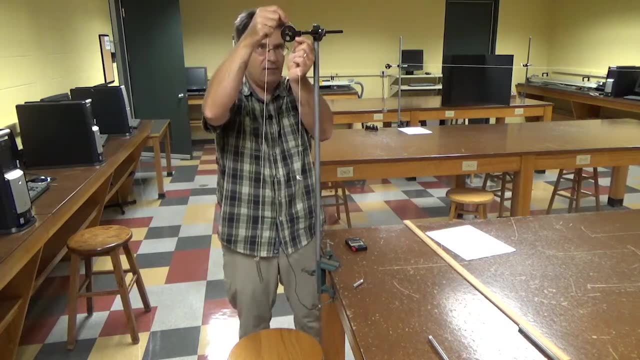 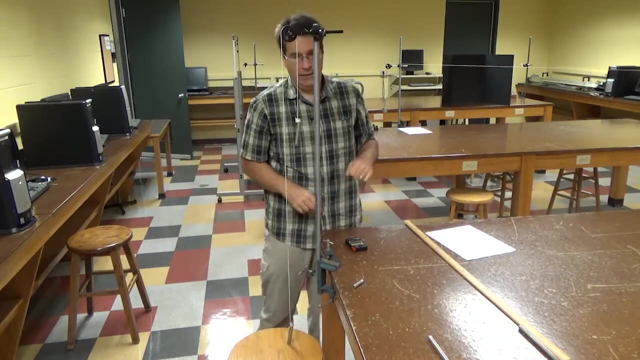 And I'll replace this guy with the 100.. So I still have 10 grams of difference, right? I think it's going to take the same time for these two objects to exchange positions. okay, And I think you'll see. now I don't have the exact same height difference because the cylinders 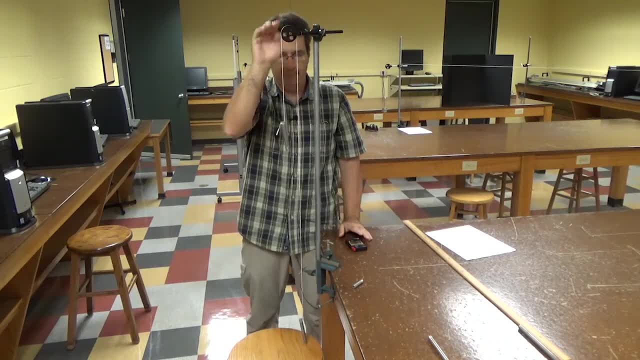 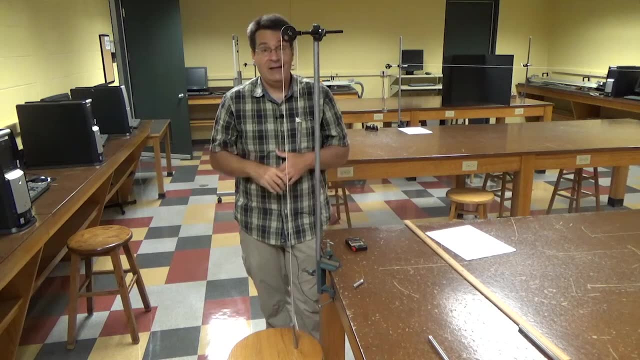 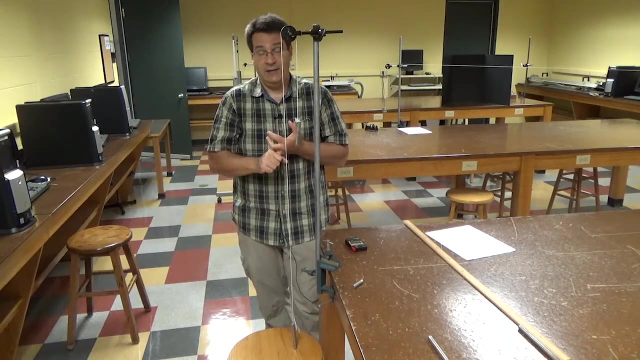 are different height, but I just want to show you that I think you can see in the video that that's definitely slower, okay, And that is confirmed experimentally. So you'll be given data for 40-50 gram machine, the 90-100 gram machine and the 190-200 gram. 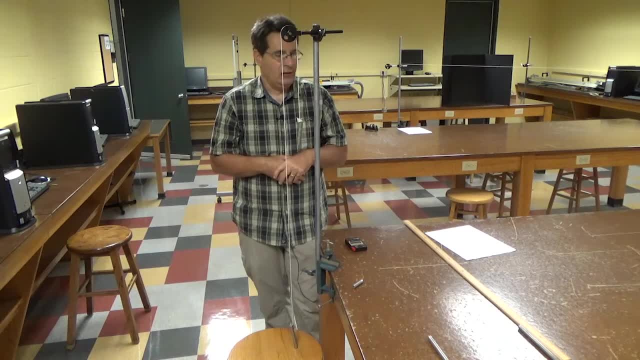 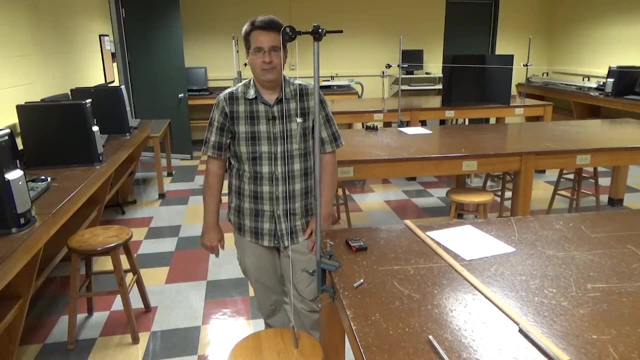 machine. okay, just so you can do some calculations using both force acceleration and conservation of energy. But we'll go through the analysis in the video and then you can complete the worksheet. Bye-bye.